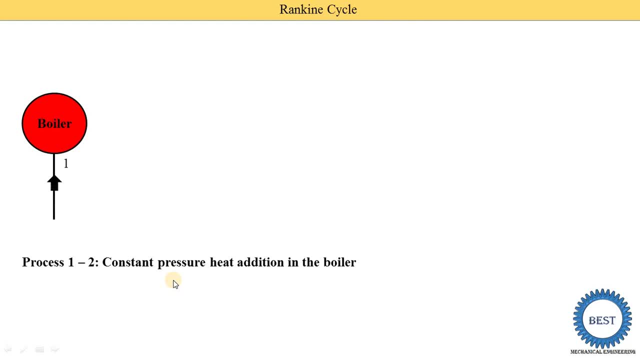 So in a boiler we supply the water from the feed pump and this water is absorbed. the QS quantity of the heat energy, Q means heat and S means supply. Okay, And this water is converted into the steam, So it is called as the process one to two. The water is heated at the constant pressure P1 in the boiler until the saturation temperature is reached. 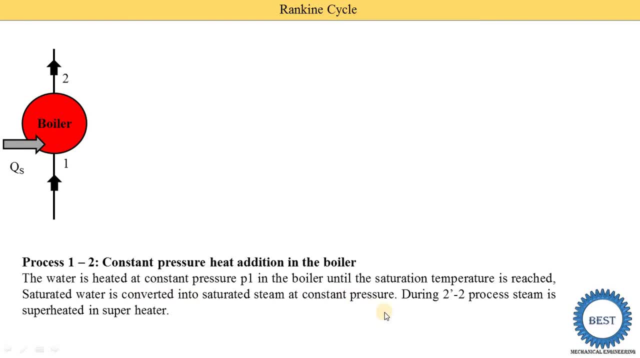 So saturated water is converted into saturated steam at the constant pressures. So in this process, you see that is a at the inlet of the boiler. one condition at the outlet of the boiler, two condition is there. Okay, So pressure remains constant. means this: P1 and P2 are constants? Okay, So when we draw the process on the PV diagram, it's coming to the horizontal lines. Okay, Now, during two days to two process, the steam is superheated in a superheater. that I explained on this PV diagram. Okay, 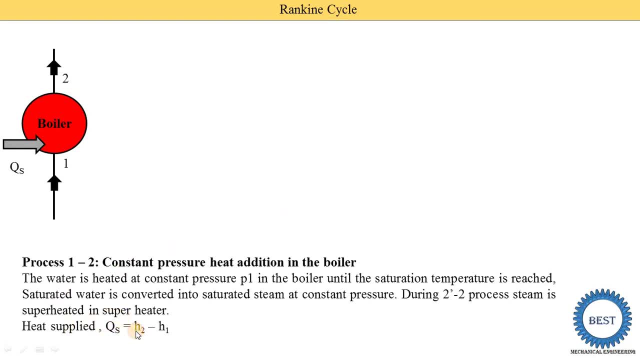 And the heat supply value is: find out. that is, a QS is equal to H2 minus H1.. So first we draw this process on the PV diagram. on the Y axis, pressure is there. on the X axis, volume is there, And in this PV diagram one curve is drawn, It is called as the saturation curve. Okay, In this saturation curve this point is called as the critical point. Okay, And from the critical point the line left side is indicate saturated liquid line, means this line is indicated, It is a saturated liquid line, means it is point. 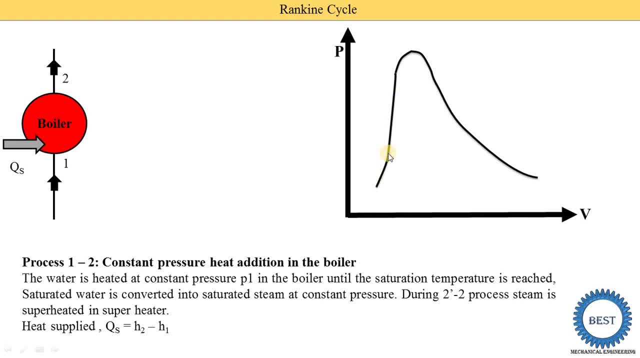 Okay. So suppose we take here point It's indicate the water. Suppose we take the point here It's indicate the water means in this line the we putting the point that is the water, Okay, Means liquid and the right side from this critical point- This is the critical point- means right side means this line is indicate the saturated vapor means any point on this line It's a indicate the vapor states Okay, And these region is indicate the superheated region. This region means region right side to the saturated vapor. 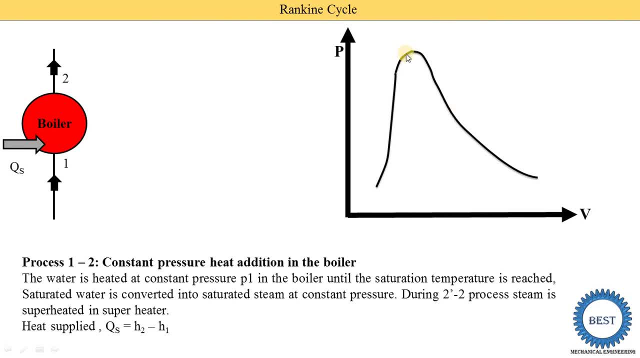 Okay, indicate the superheated region. same way, region left side to the saturated liquid line is indicate the saturated liquid and the area under this cow line is indicate the mixing of liquid plus vapor. so it is called as the wet regions. okay, so where is the point number? 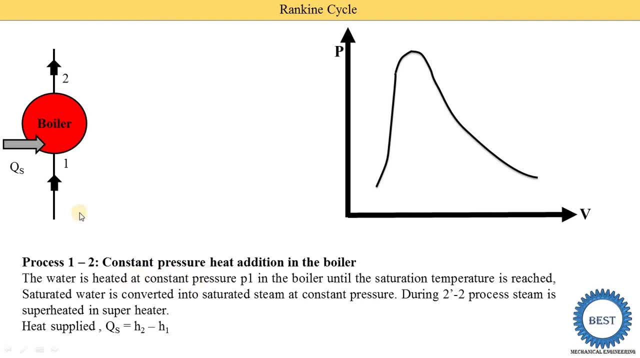 one is coming, so we know that it is a constant pressure process. okay, at the when the water is entering the boiler, it have the high pressure, means point number one is coming in this upper region. okay, because here the value of the pressure is zero when we moving in upper direction. 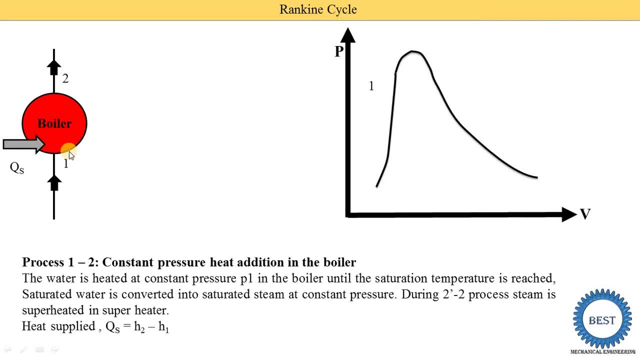 the pressure is increased. okay, so we know that at the entry of the boiler the state of the working substance is the liquid. means point number one is coming somewhere here on these lines, or either the left side of this line. okay, and this water is converted into the vapor. means it is converted into the steam. means point number two is coming. 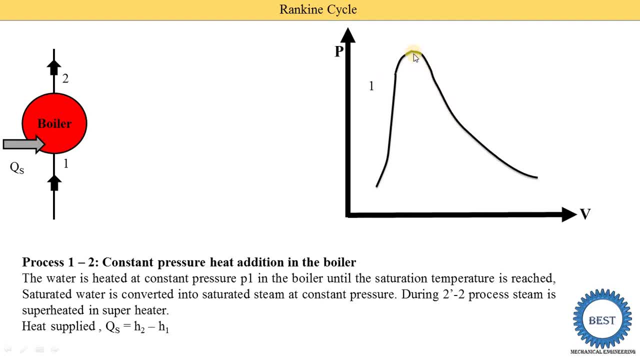 on this higher region but on this right side line, because from the critical point line is indicate the vapor. Okay, so point number two is coming here. okay, so this is the complete line, that is a 1 to 2. okay, so here at the two days point, this point is indicate two days. at this point it. 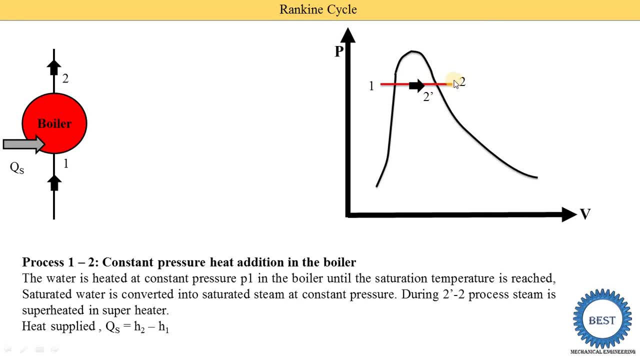 is the saturated steams okay. and at the two point is indicate the superheated means the any point right side to this saturated vapor light is indicate the superheated okay. so here we mentioned during the two days to two. so this is the two days point and this is. 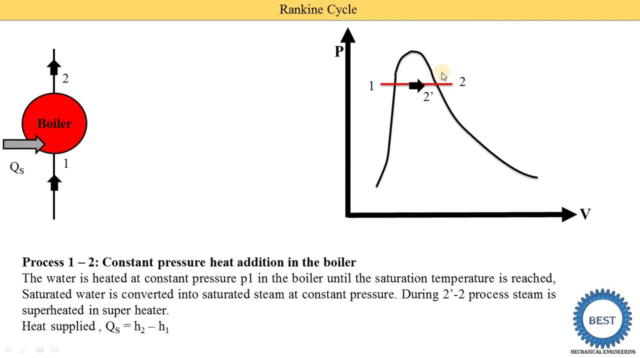 the two point These process. this steam is superheated in the super heater means from the boiler the steam is coming, is the saturated okay, but we need to convert this saturated steam into the superheated. we require the superheater. so this is the point number two. 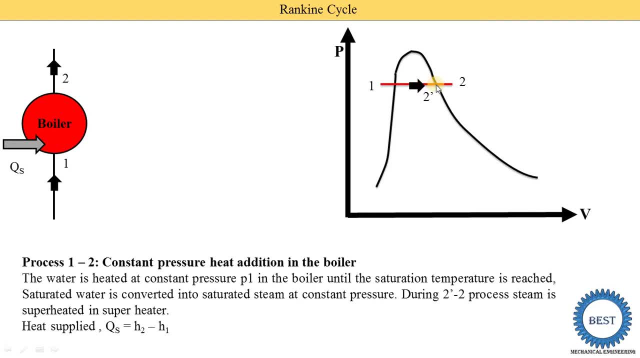 so we can draw the point number two anywhere. okay, that is a two days point here or a two point here. same way, one point is coming also on this lab point, or either it is also coming this: saturated liquid lines. okay, it is, depending on the conditions and what amount of the heat is added. 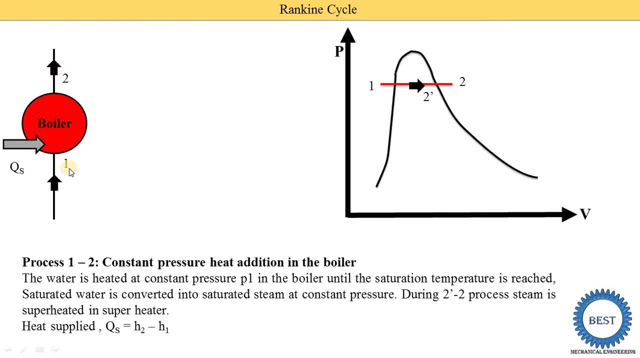 so when we hear at the heat this h2 is higher than the h1, so it is be written that is h2 minus h1. now the second process. it is the process 2 to 3. it is the isentropic expansion in the turbine. 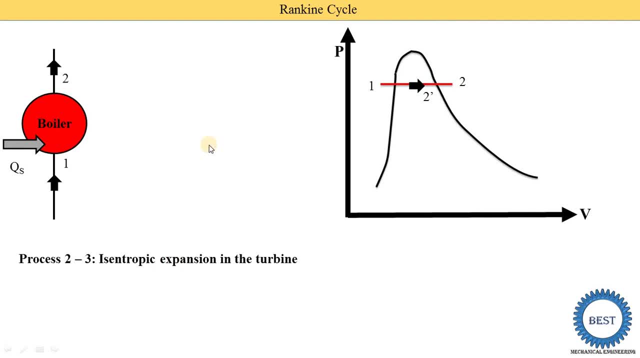 means second component is the turbine, okay. and isentropic expansion means isentropic means entropy remains constant during the expansion process. okay. so when the expansion is done, what happened? the pressure is reduced means high pressure is reduced pressure. high temperature, superheated, dry, saturated or a wet steam generated in the 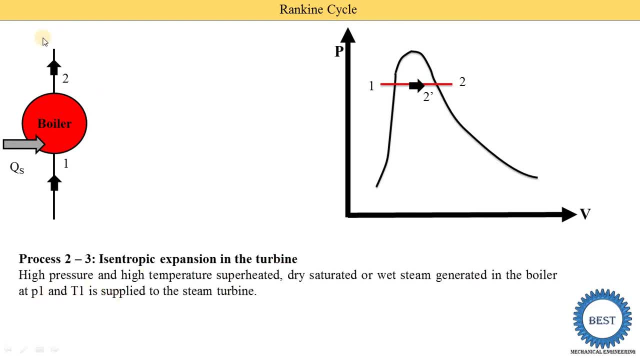 boiler at the p1 and p1 is supplied to the steam turbine, means at the point number two, that is, a high pressure, high temperatures, superheated steam is there, or a dry and saturated or a wet steam is there? okay, means it is. depending on that means, suppose there is two, two point. 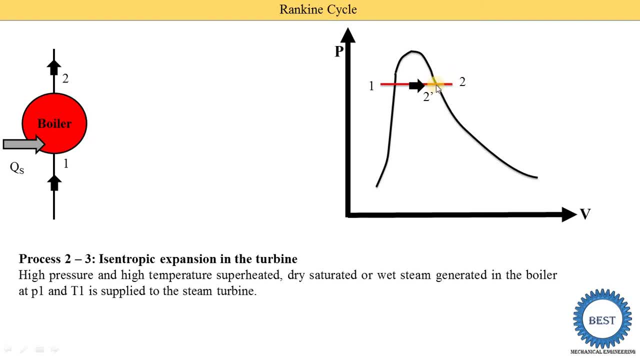 is here that is indicated it is a superheated steam. suppose it is two dash. point: it is indicated dry and saturated and suppose wet steam is that, and this point is coming here under this wet region means any steam is there. okay, it is supplied to the boiler at the p1 and t1. 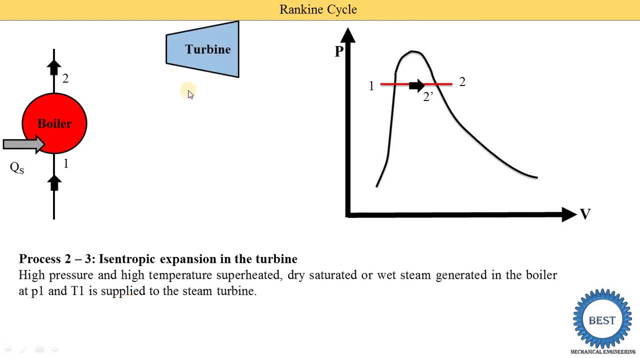 is supplied to the steam turbine. so here this turbine is there, not, it is p1 and t1, but it is a p2 and t2 means here the two point is there, okay, and at the three point the steam is coming out from the turbine and this turbine is produced. on work done and this work done. 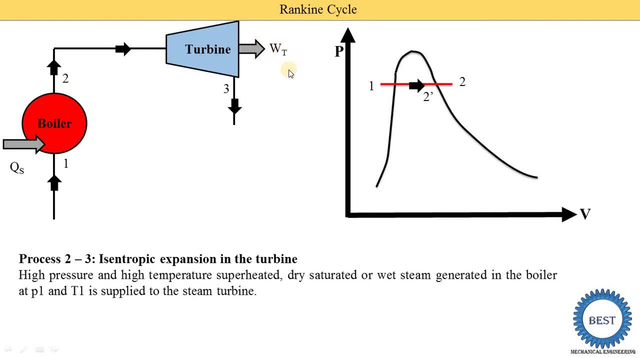 is denoted as the wtf. That is, a w means work and t means turbine. steam is expand isentropically means entropy is remains constant during the expansion process. okay, so this steam is expand isentropically into a steam turbine up to the condenser center means during the expansion. we know that the 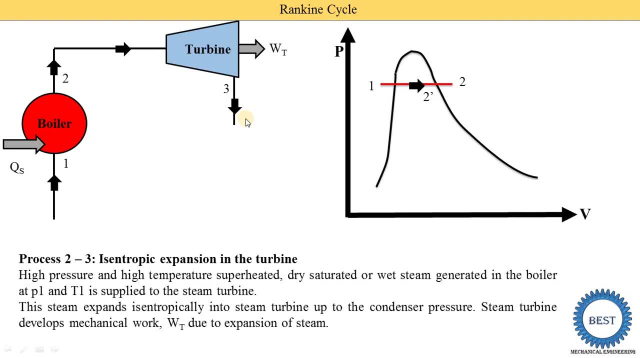 pressure is reduced and the volume is increased and the entropy remains as it is. steam turbine developed mechanical work wt due to the expansion of the steam, so turbine work wt is going to is equal to h2 minus h3. okay, now how we draw this isentropic expansion line on this pv diagram. 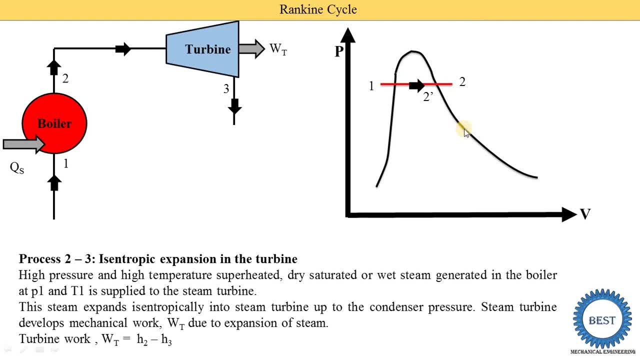 okay, so we know that the pressure is reduced, means point number three is coming on the below side to the point two. okay, and we know that volume is increased. then the point number three is coming right side to the point number two. okay, so point number three is coming somewhere here. 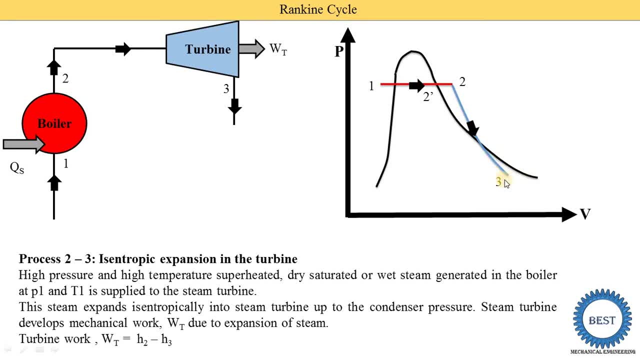 it is the point number three. so here the it is the weight region. okay, so it is not necessary that the steam outlet from the turbine is the weight steam. it may be dry and saturated, it may be superheated, depending on the condition. means point number three is coming either in weight. 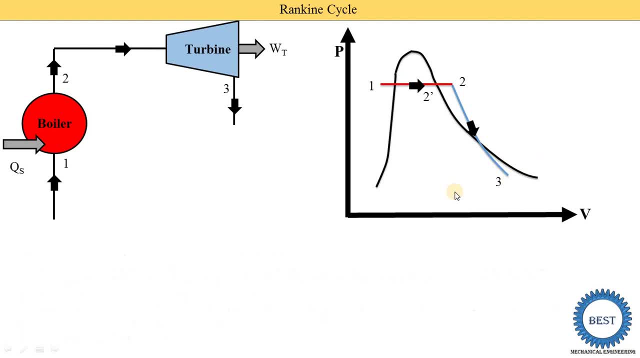 region on these lines or at this line, depending on the types of turbines and depending on the process and the turbine work is the h2 minus h3. then after the third process, it is the process three to four. it is the constant pressure. heat rejection in the condenser means the third. 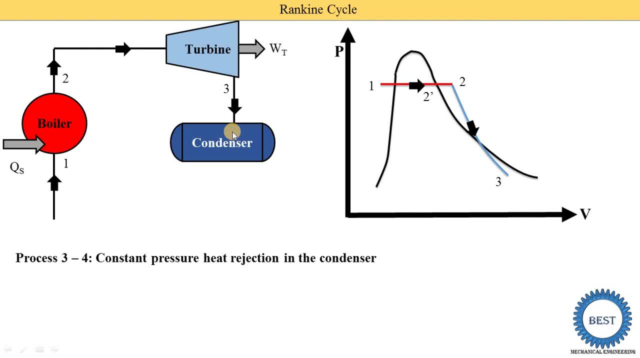 component is the condensers. okay, so condenser is a one type of heat exchangers, so okay, and it is used to reject the heat to the atmosphere. here we also mentioned that is a heat rejection process. okay, so you simply remember that the heat addition in a boiler qs and the 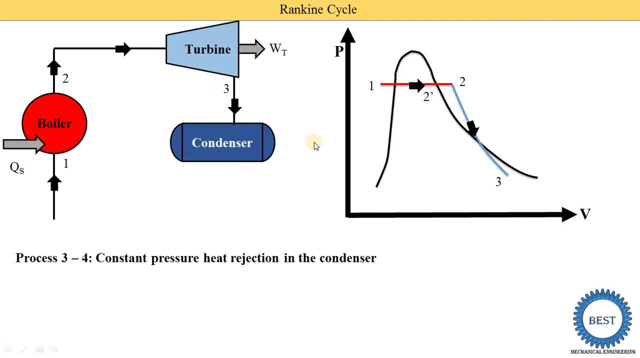 heat rejection the condensers are occur at. the constant pressures means we need to draw the horizontal line. okay for this. one to two process in the boiler and process three to four in the condensers. the exhaust steam from the turbine enters into the condenser. here you see the 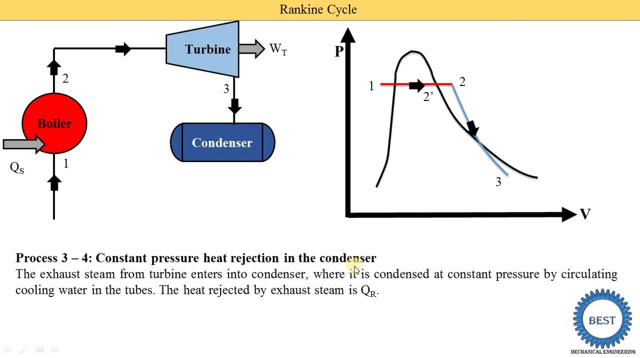 steam coming out from the turbine is supplied to the condenser, where it is condensed at the constant pressure by circulating the cooling water into the tubes. the heat rejected by the exhaust steam is denoted as the qr. okay, so in this condenser, number of tube is there, okay, and the cooling water is required. so you know what is. 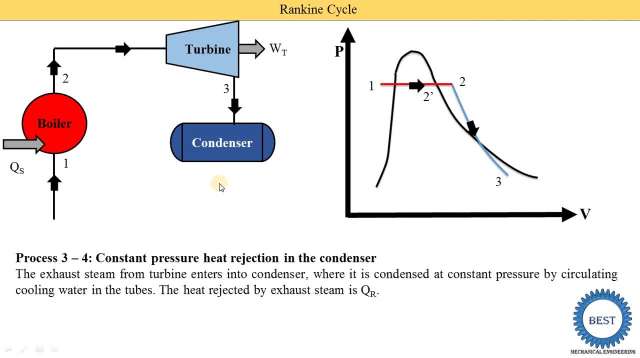 the meaning of condensed process, condensation. condensation means the steam is converted into the water. it is called as the condensation process. that why its name is given: the condenser. and in this condenser the steam is converted into the vapor at the constant pressure. okay, so in this condenser point at once, we know there has to be a styrofoam beneath the. 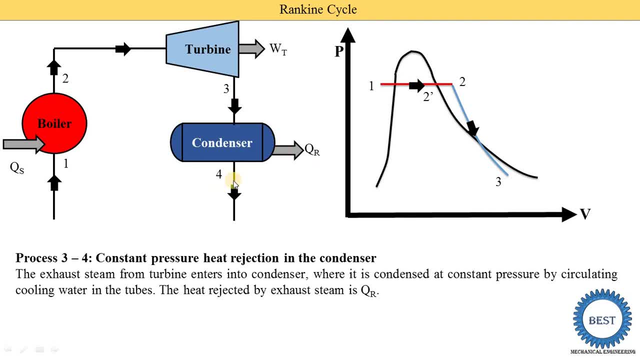 condenser water in order to sip of this liquid, of this liquid will be entered into this temperature system the whole of the denuded process that we will be using, entonces de caelo vapor line. so we know that at the outlet of the condenser water is there, so means point number. 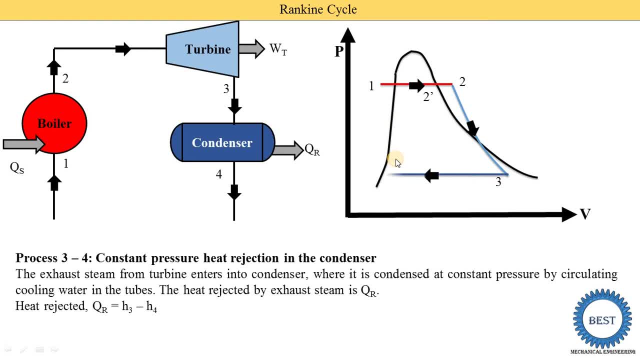 four is coming on this line. okay, so it is the this line, so it is a point number four, okay. and how amount of the heat is rejected? how we find out? so heat rejected qr is the h3 minus h4. now the next process is the process four to one, that is, isentropic compression in the pump, or it. 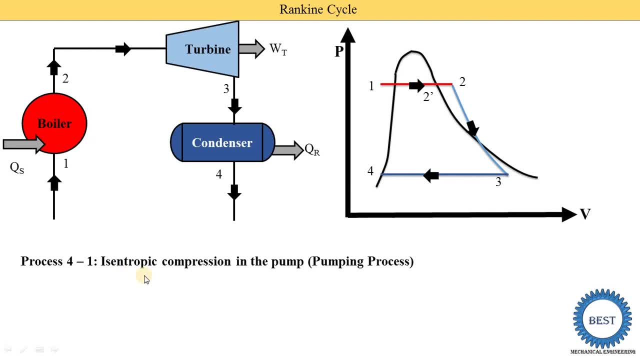 is called as the pumping process. isentropic means the entropy is remains constant. compression means the pressure is increased and the volume is reduced. but in a pump what water is there? so water volume is not reduced. okay, so we need to draw these one vertical lines and the isentropic. 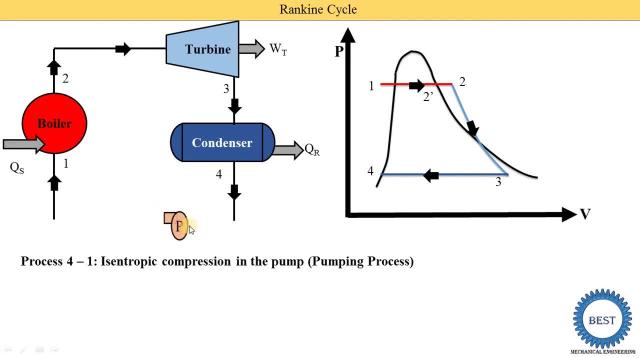 means entropy is remains constant and the pressure is increased. so here we putting the component pump. the condensed water coming from the condenser is pumped into the boiler at the boiler pressure with the help of the feed pump means here the lowers pressure in these condensers okay, and the boiler pressure is higher. 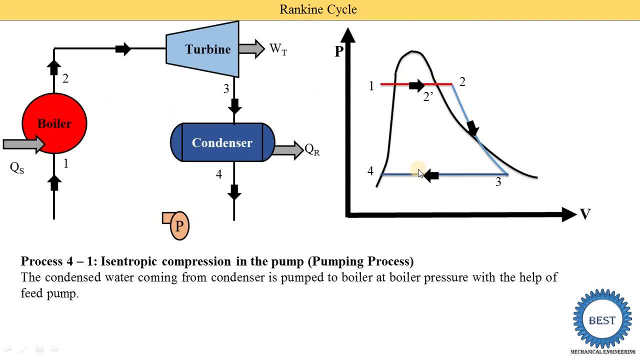 here you see that, the one, two, two, it is boiler line, so here the higher pressure, and at the entry of the pump it is the lower pressure. so function of the pump is to increase the pressures. okay, so here you see it is. the water coming out from the condenser is supplied to pump. its pressure is. 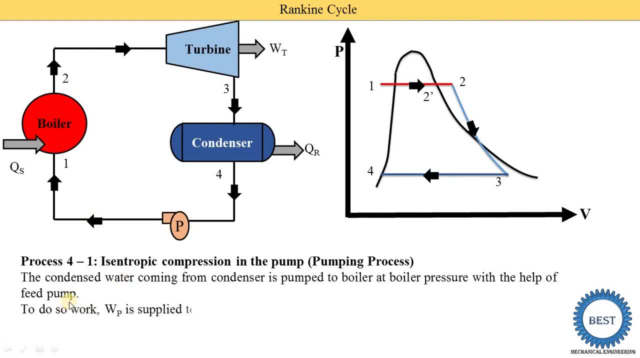 increased and it is supplied to the boiler to do so. to do this increase the pressures, we need to supply some work done. this work done is indicated as the WP quantity of the work done. so WP is supplied to the feed pump, so pumpwork is denoted. WP is equal to h1 minus h4. so how we drew this line on this pv diagram, so it 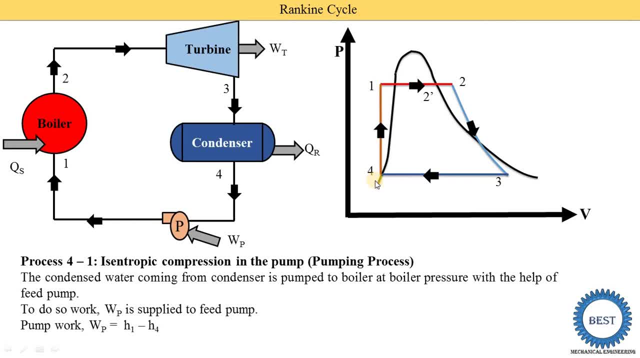 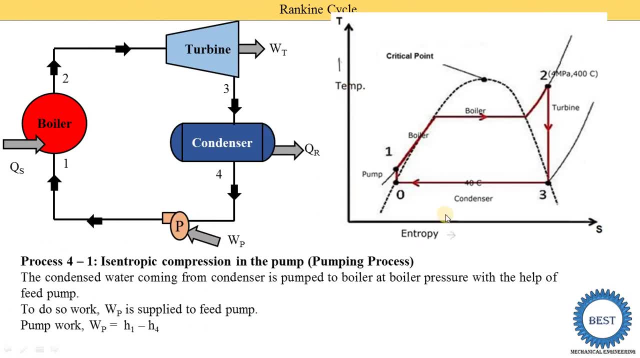 is just go to the simply vertical line. so here you see this: the pressure is increased from p4 to p1. now we draw the t-s diagram. okay? so here you see, this is the t-s diagram. okay, now, that is the same type line. this is the critical point. left side is indicated. 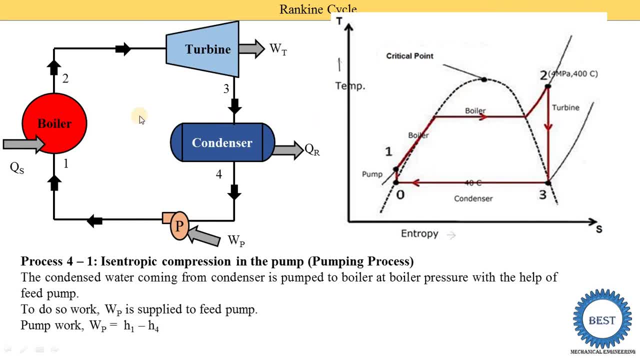 liquid. right side is indicate saturated vapor line. so point number one is: draw here. okay, so it is. the liquid line means its temperature is increased first, okay, this means sensible heat, then after, at the constant temperature, at the constant temperature its phase is changed from water to vapor and then it is go to the superheated means. this line is indicate, it is the constant. 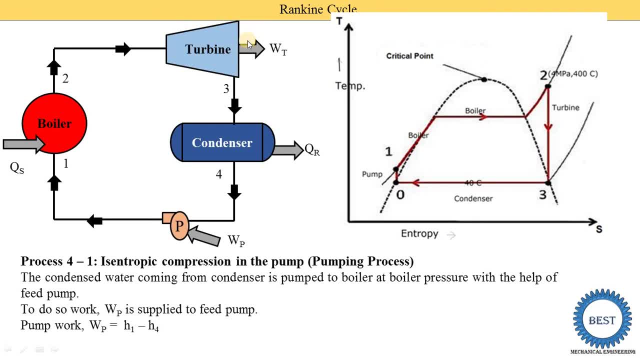 pressure line, okay. second process, that is, isentropic expansion means entropy is remains constant. so here, on the x-axis, entropy is there. okay, means s2 is equal to s3. so here we take the projection of the 2 to 3 line. okay, what we did. x2 is equal to s3 means we need to draw the vertical. 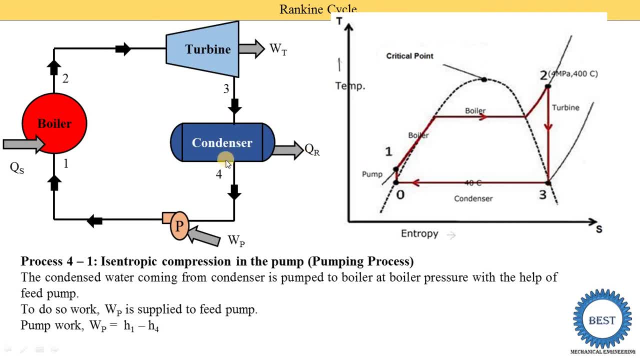 line. okay, then after 3 to 4 is the condenser, means the steam is converted into the water. so we need to draw this type line and this process is done at the constant temperature, but its phase is changed, means that is a latent heat rejection is there. then 4 to 1, it is the pumping. so here 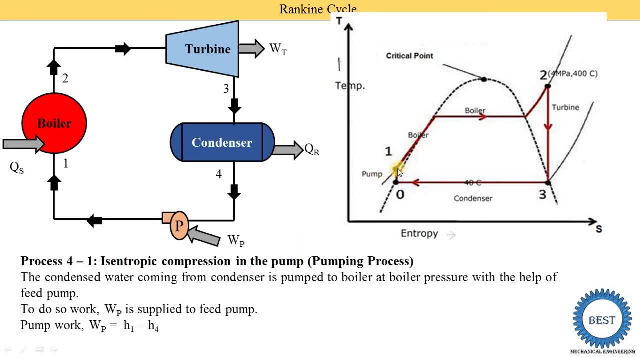 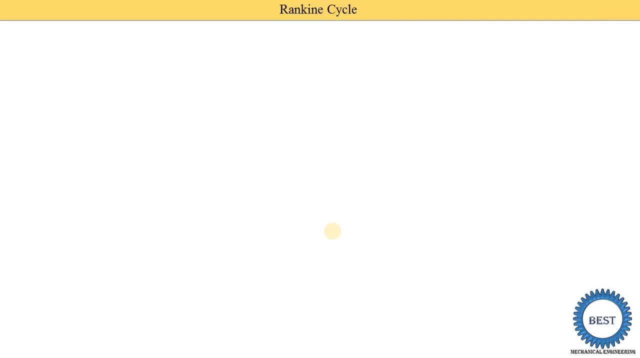 we draw this pumping line, so it is also isentropic, means we need to draw the vertical line. okay, so this is the pv and ts diagram. understanding now we find out the efficiency for the rankine cycles. before moving ahead, i request to like the video and subscribe my channels for watching the more 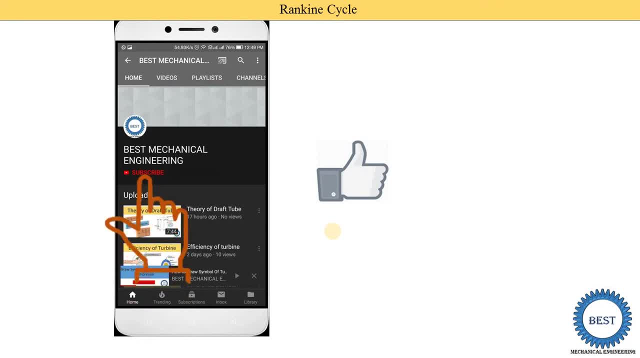 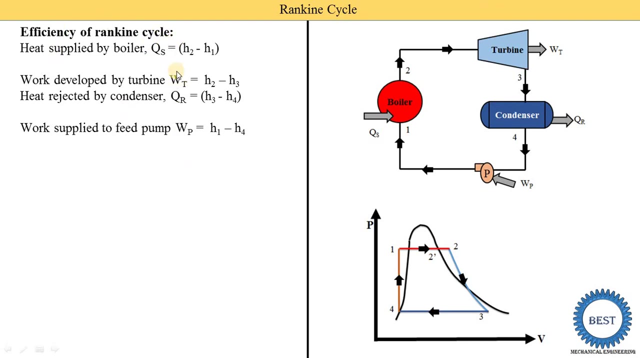 video related to the bme subject or power plant engineering. okay, for other subject, the, i request to visit the playlist for the bme subject. the various link is provided in the descriptions as well as in a card, so we take these equations. okay, we already discussed this equation, that is, a heat supplied. 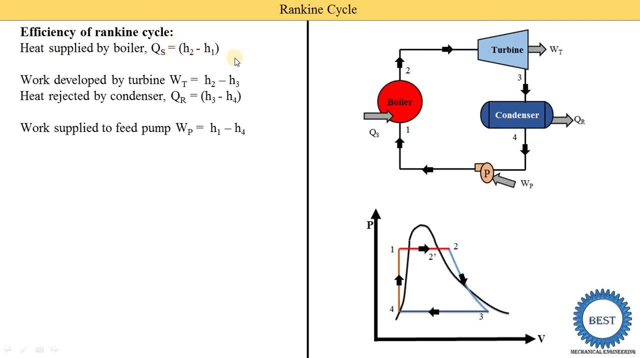 in boiler. so qs is equal to h2 minus h1. so somewhere- you see, here the outlet point minus inlet point is written h2 minus f1, because here the one input is there, second heat input is there, means this value is higher. okay, two value is higher. that's why we mentioned h2 minus h1. 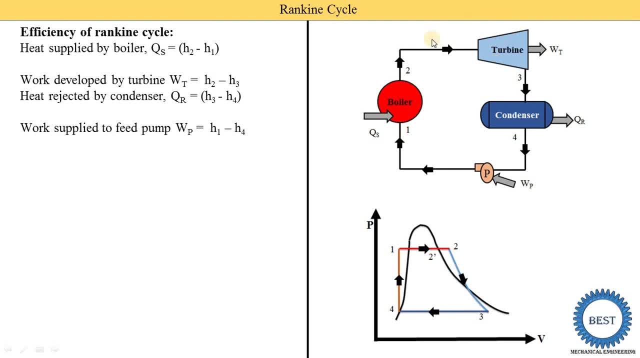 in a turbine the steam is, loss is energy. okay means the value of two is higher and some work is output, so it's enthalpy. at the three point is reduced. same way heat is rejected from this three point means h4 is lower. that's why it is f3 minus h4 is written in a pump. we had some work done so 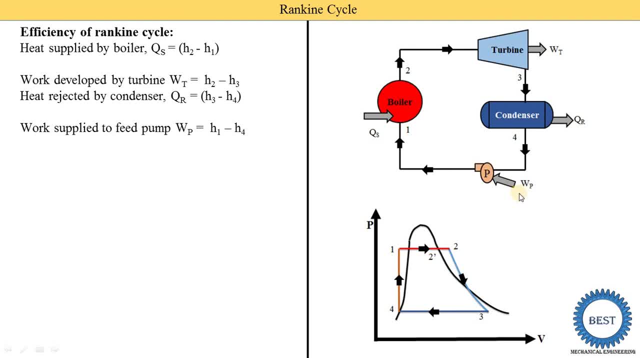 here the h4 is coming, and in this h4 we add some work means h1 is higher. that's why here the h1 minus h4 is mentioned. now we find out the network developed. so network developed is denoted as the w net okay means what work is produced and what work is supplied. so here you see, in this diagram, 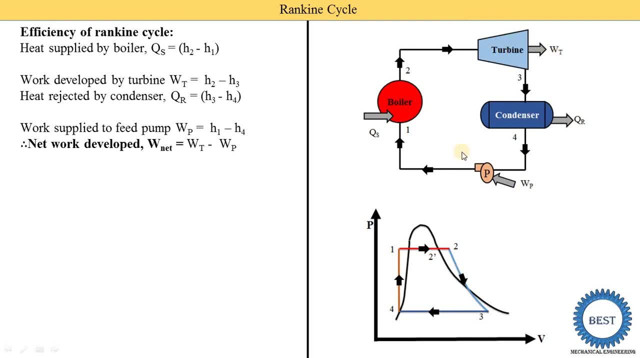 turbine is produced some work done and in a pump we supply some work done. so wt is positive. when the system is produced work done, it is denoted as the positive. when we supply bulk done to the system, it is indicate negative. so it is the wt minus wp. so we have the value of wt that 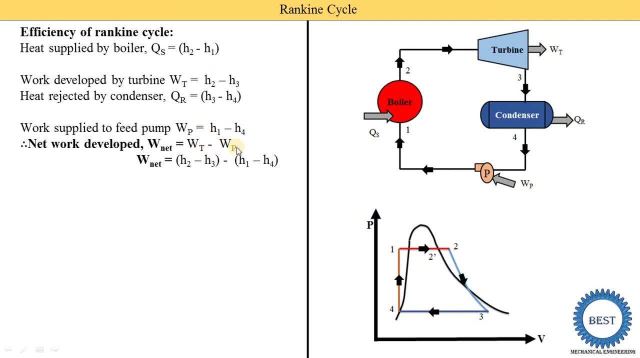 is h2 minus f3, we have the value of wp. that is h1 minus h4. now what is the equations of the efficiency? so efficiency of the rank and cycle is denoted by these symbols. okay, so network developed by heat supply in the boiler means what is the output and what is the input. okay, so in the rank, 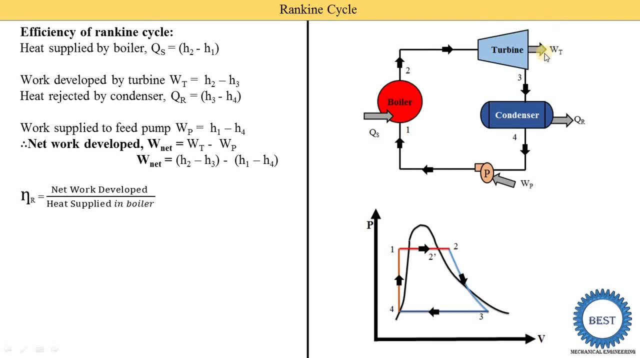 and cycle, or the steam power plant. the output is the wt, but at the same time we supply some work done to the pump. so we consider network then, and input is the heat energy supply to the boiler. that is the us. so we have a network developed that is h2 minus f3 minus h1 minus h4, divided by heat supply. 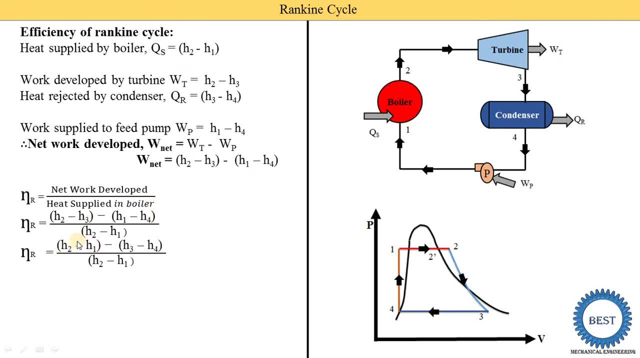 that is h2 minus h1. now we do the small correction in the upper part of this equation. that is h2 minus h1 means this h1 is coming in these sides and this f3 is supplied on these sides. okay, so it is written h2 minus h1, minus another bracket, h3. 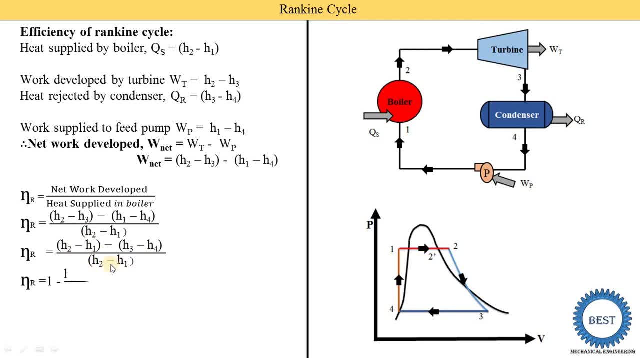 minus h4, divided by h2 minus h1. now we divide this equation in the two parts, that is h2 minus h1 divided by h2 minus h1. so this f2 minus h1 is cancelled. so we return 1 minus f3 minus h4 upon. 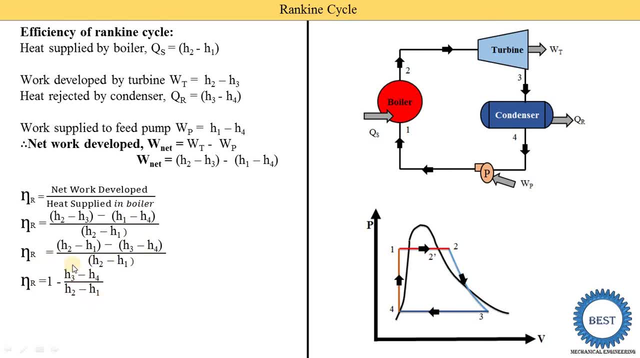 h2 minus h1. so this is the equations for the rank and cycle efficiency. now, what is the f3 minus h4? so here you see, this is the heat rejections. okay, so instance of this f3 minus h4. we are also written: this is the qr. what is h2 minus h1? so you see, it is a heat supply. okay, so rank and 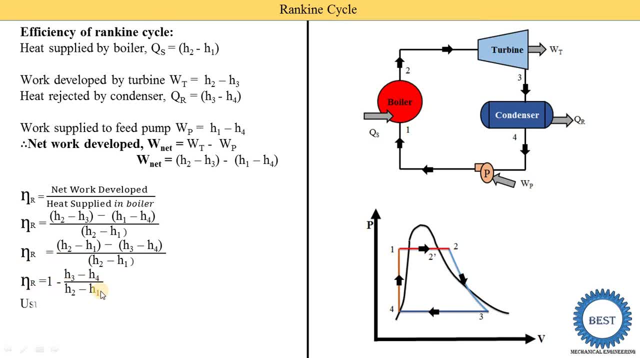 cycle efficiency is one minus qr upon qs. now suppose we neglect the power. so usually powper is very small, hence it is a negative, or we can neglect it, not negative, but we can neglect it. so when we neglect the power, okay means only the turbine is work, is our output. so in upper part turbine work is there. that is h2 minus f3 and heat supply. that 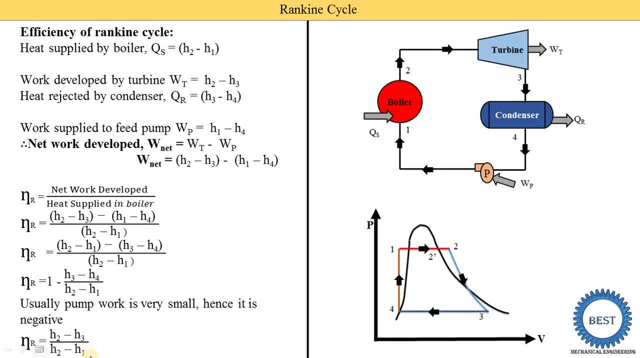 is a h2 minus h1. okay, so this is the final equations for the efficiency of rankine cycle: this equation of the efficiency when we consider the pump work and this equation is when, when we neglect the pump work. so thank you for watching this video. if you learn something, then like the.